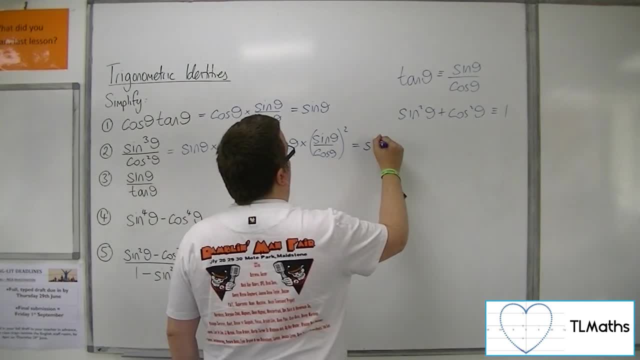 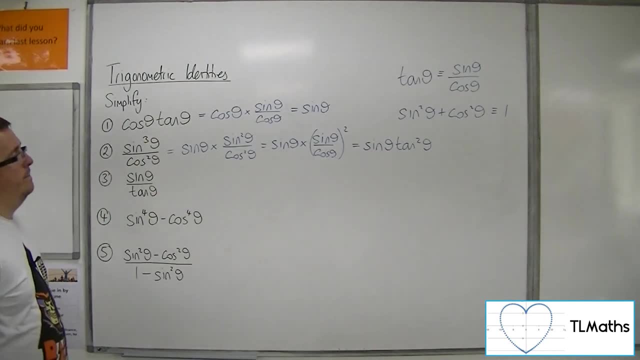 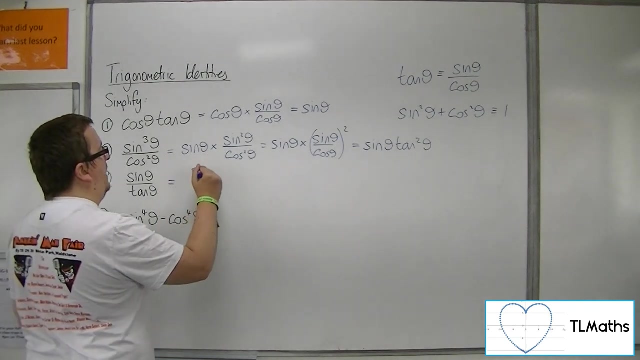 Sine over cos we know is tan. So this is the same as sine theta times tan squared. OK, And that's really where you probably leave that one. OK, That's as far as we can really simplify it. Number three: sine over tan. Well, we know that tan is sine over cos. 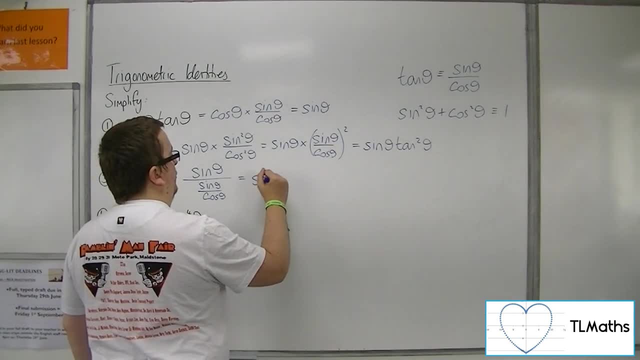 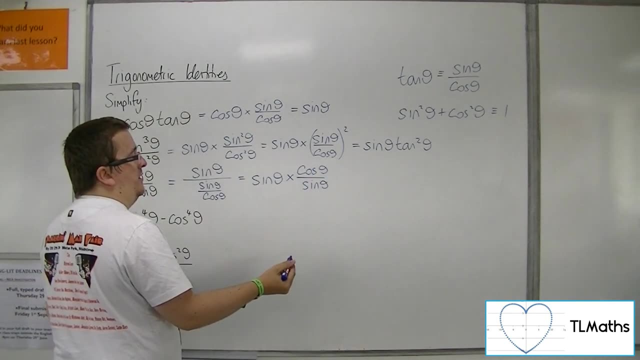 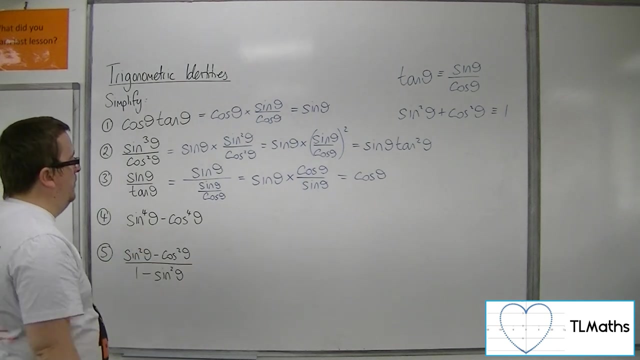 And we know that when we divide by a fraction it's the same as multiplying by its reciprocal. So here the sine thetas will cancel and you just get left with cos theta. Now, sine to the 4 theta, minus cos to the 4 theta. 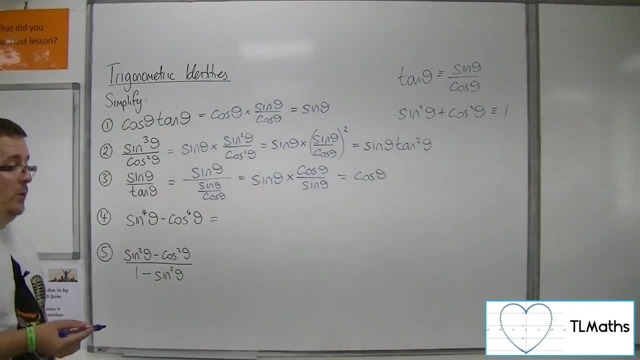 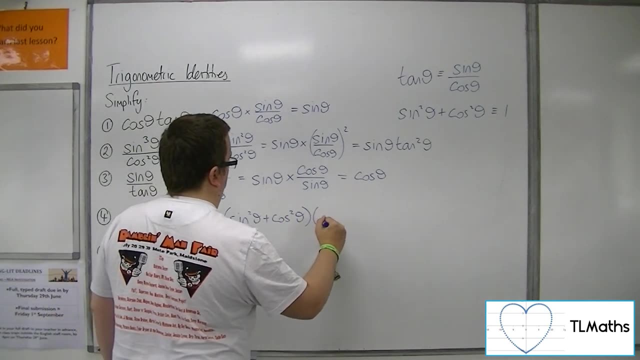 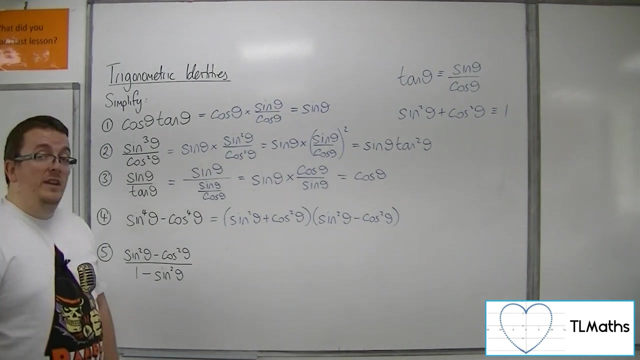 Well, that is actually the difference of two squares, So you could write that as sine squared theta plus cos squared theta. times sine squared theta minus cos squared theta. OK, Now the sine squared theta plus cos squared theta we know is 1.. 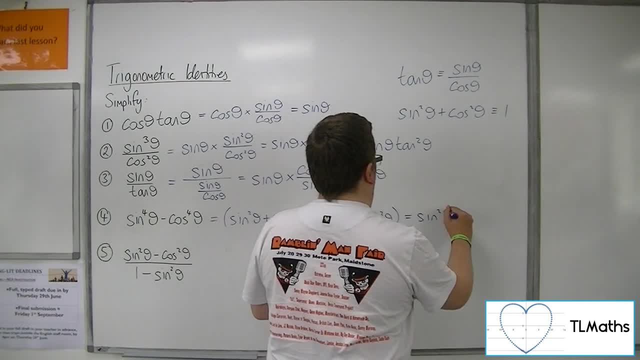 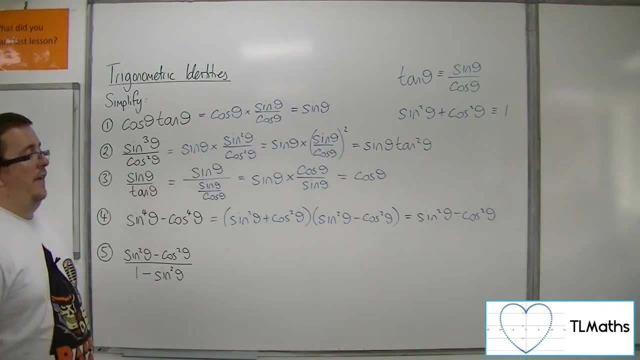 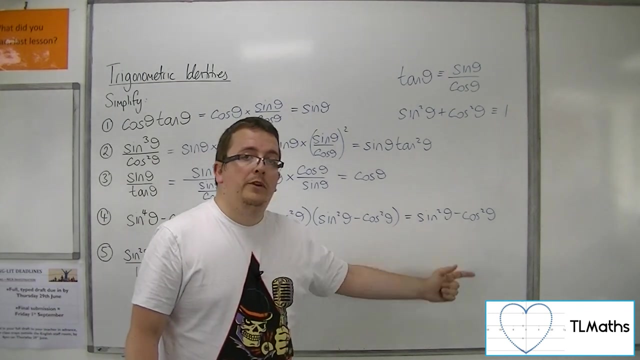 So this is just 1 times sine squared theta minus cos squared theta. Now, we can't really go anywhere further than that. OK, But it's showing that sine to the 4 theta minus cos to the 4 theta is actually the same as sine squared theta minus cos squared theta. 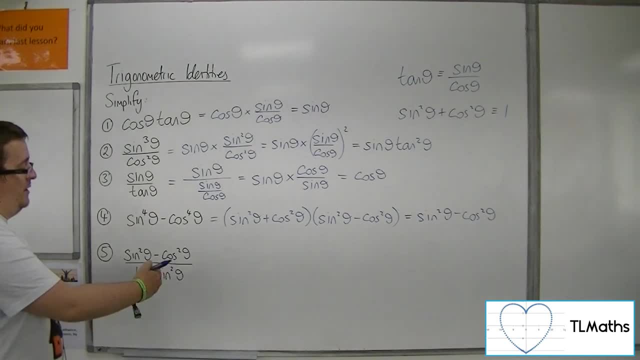 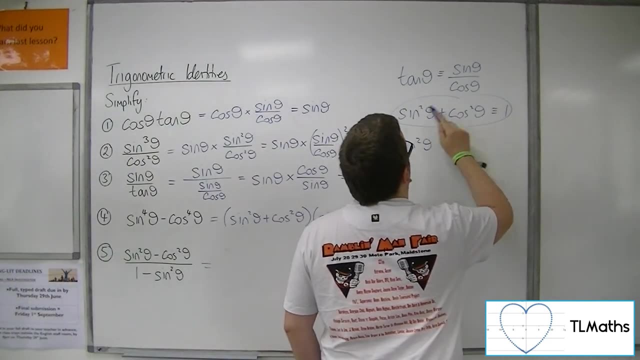 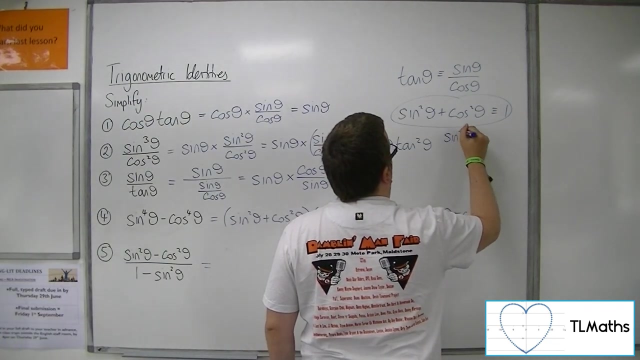 Now, sine squared, theta minus cos squared, theta over 1 minus sine squared. Well, from that second identity here, right? what you can then say is that if you subtracted cos squared from both sides, that sine squared is 1 minus cos squared. 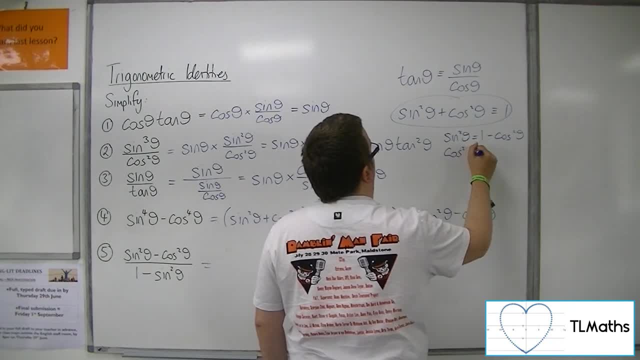 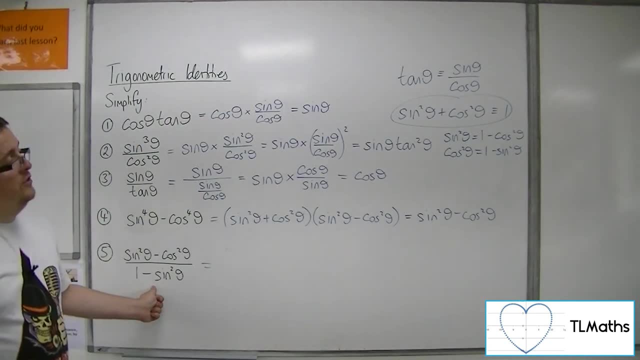 Or if you subtracted sine squared from both sides, cos squared is 1 minus sine squared. These are very useful to remember So that when I notice I've got a 1 minus sine squared I can replace them. And I can replace that with cos squared. 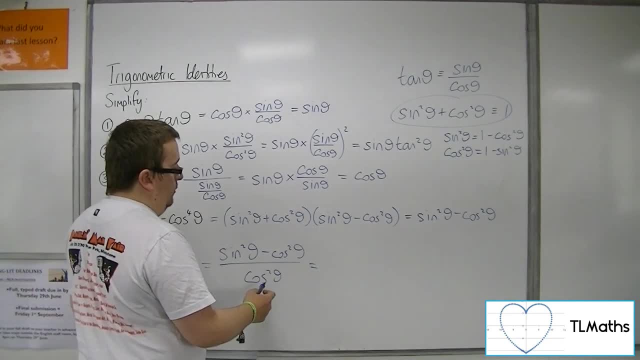 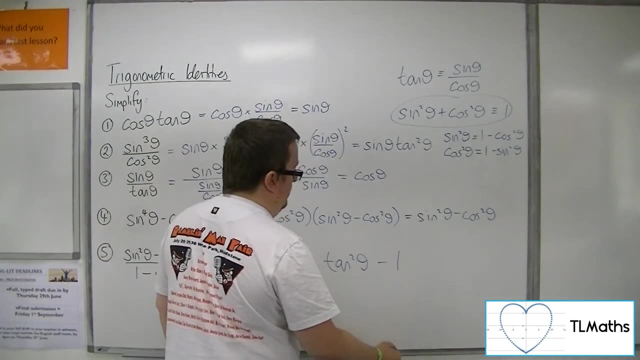 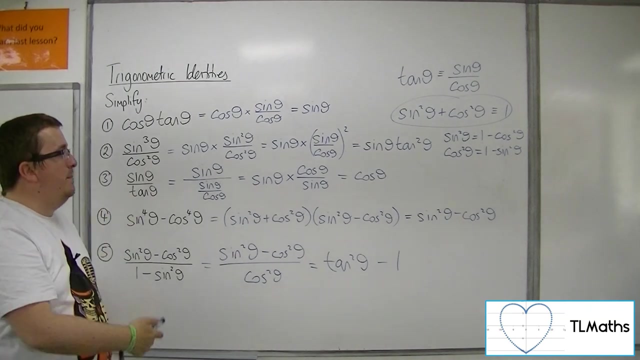 So now I've got sine squared over cos squared, which I know is tan squared, Takeaway cos squared over cos squared, which I know is 1.. So this is the same as that. OK, And that's how we can simplify trigonometric identities or trigonometric expressions. Using the trigonometric identities, The trigonometric identities that we've learnt.